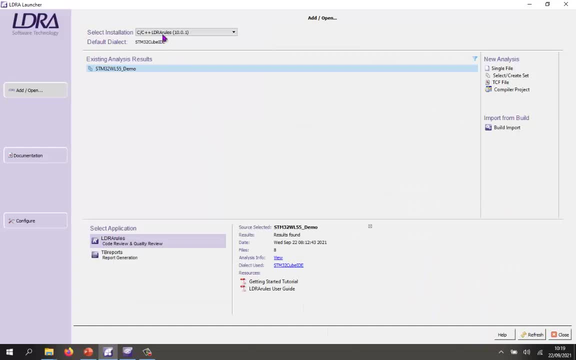 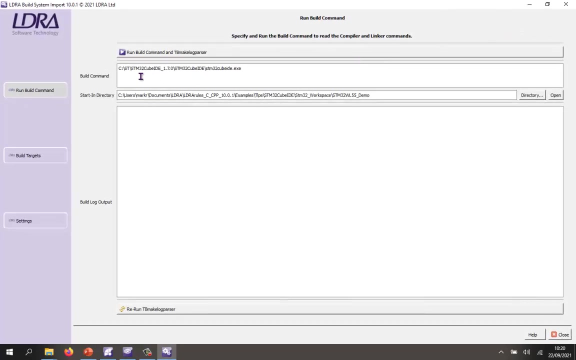 complex. Now this is the LDRay launcher, And here we can see I've selected LDRay rules and I've told it that basically, I'm going to be using the STM32Cube IDE. So what I need to do is I need to start, first of all, the build import And, inside, the build import. 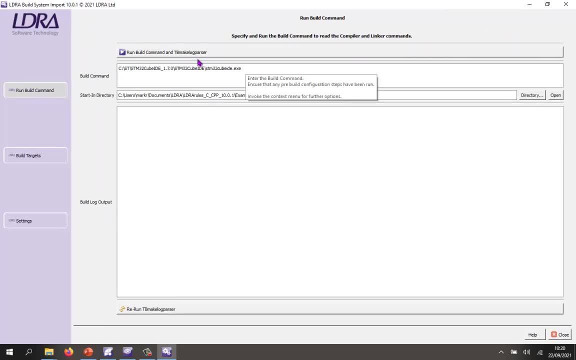 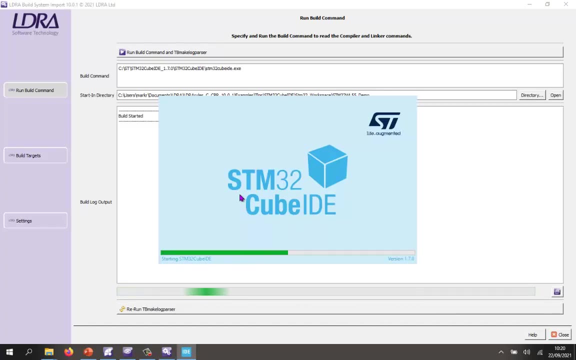 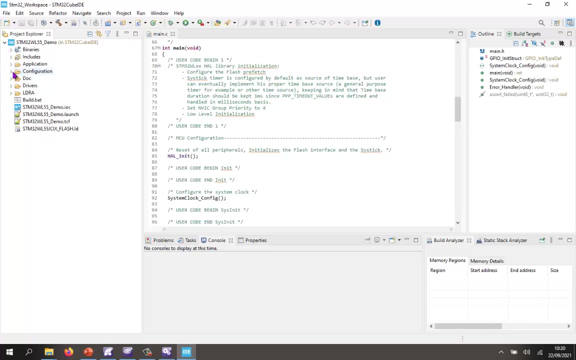 I'm going to invoke the STM32Cube IDE, So we should see this open up, And this is important, because what LDRay is going to do is it's going to listen now to everything that happens inside of the IDE, And from that we're going to be able to get an idea of what source files. 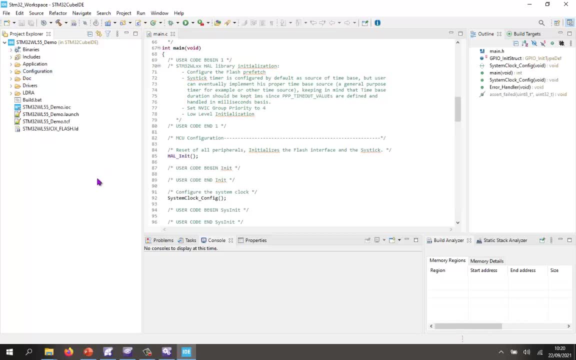 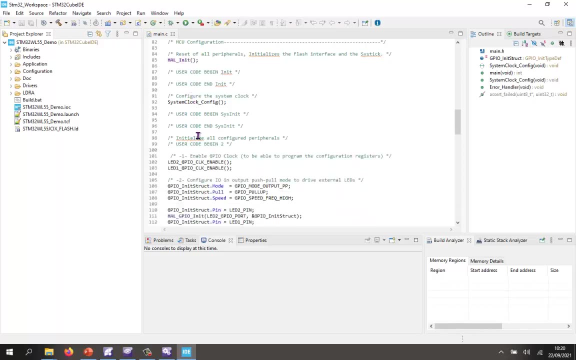 are there, what include paths, what defines, et cetera. So, anyway, here we have the program And, as we can see, there is a main here And we're calling hal init, And then we're probably going around in an infinite loop here, and 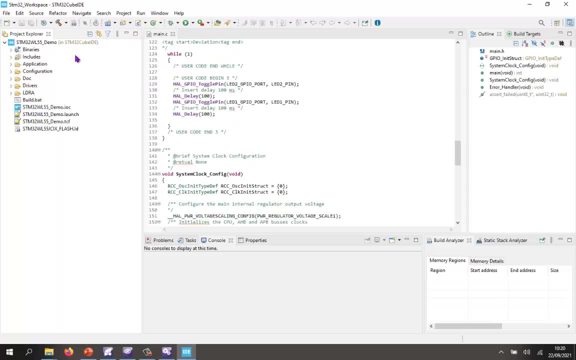 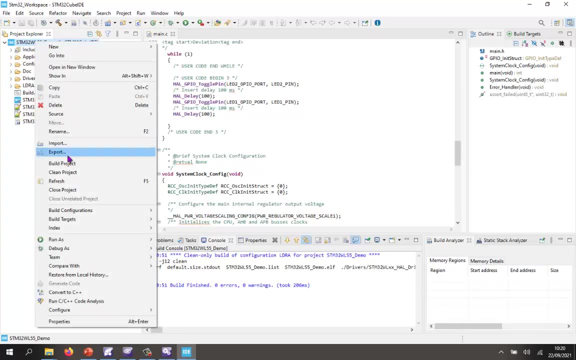 just toggling some LEDs. So, first of all, what I need to do is I need to perform a build. So I need to do a clean build. So I'm going to clean here And now I'm going to do a build. 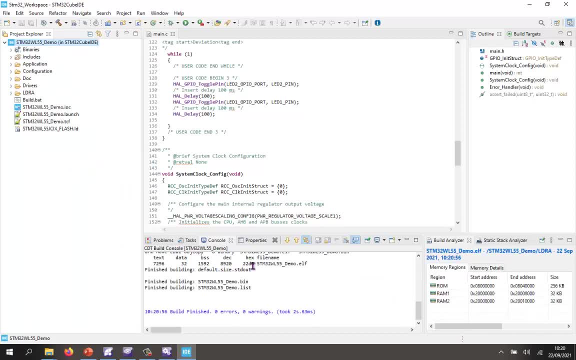 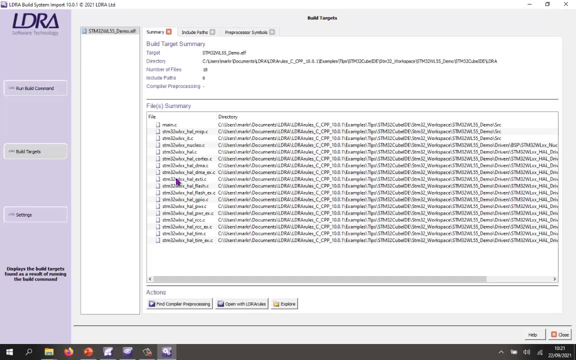 And we should see here that it's using the GCC ARM compiler And it's built this ELF file. So I can now close this down And what's going to happen is: LDRay is now going to analyze what happened And it saw that there was an ELF file that was built. It's seen a list. 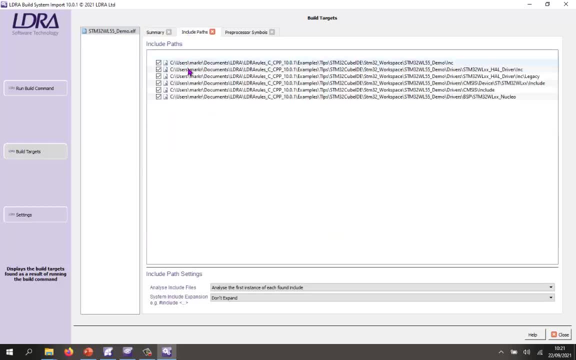 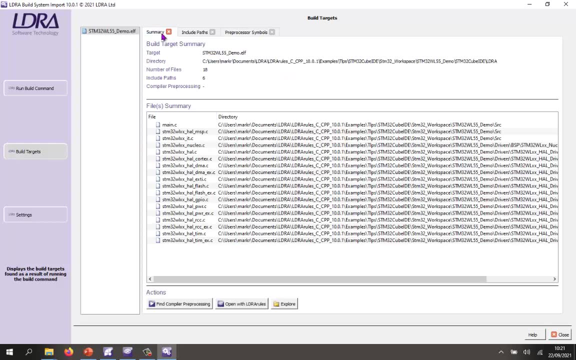 of all the source files. It's also found the include paths where it's going to find the headers, And it's also got a number of preprocessor symbols. If I wanted I could find. I could run the compiler preprocessing and find out. are there any additional defines that are? 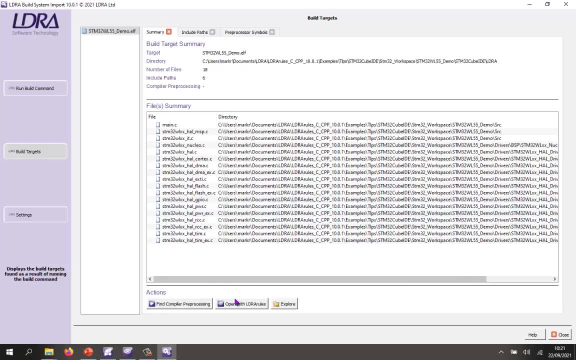 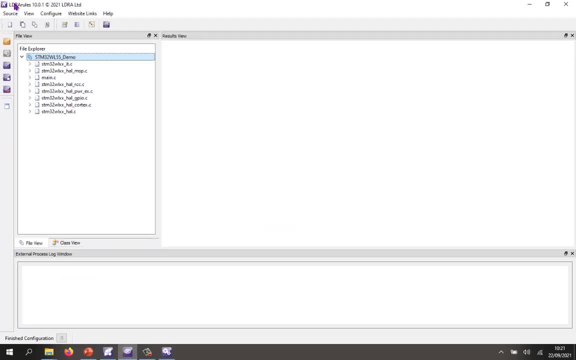 known by the compiler. So once I've done that, I could then open this with LD rules. But to save time I've already done that, And so here we have the project inside of ELDRay rules. I've also performed the analysis to save time. So first of all I can go and take a look and see. 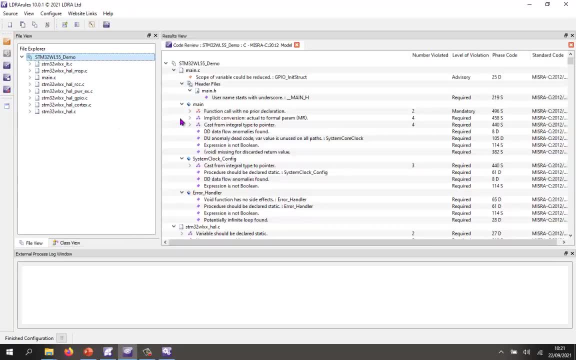 well, is this code compliant, So I've configured it to use the MISRAC 2012.. If I wanted, I could select any other standard or even create my own standard And, as we can see well, this code is not compliant. 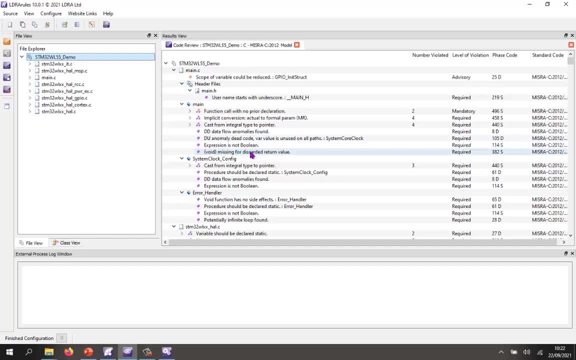 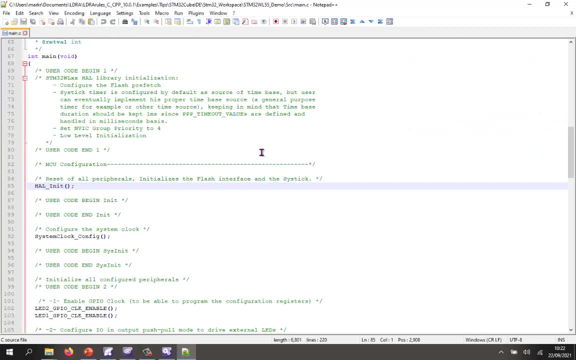 I can see we have quite a few number of violations. If I want, I could say: OK, let's take a look at this one. Avoid missing the discarded return value. Well, let's double click. This opens up my editor And there we can see we're calling halinit And imagine that halinit must return. 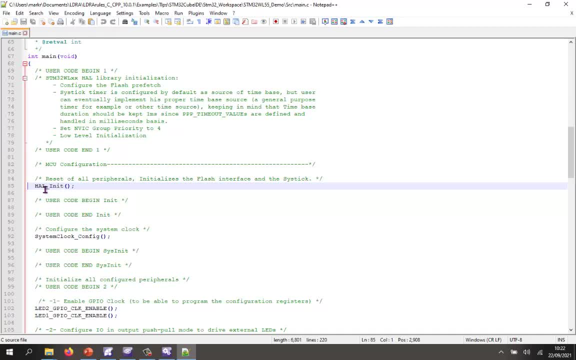 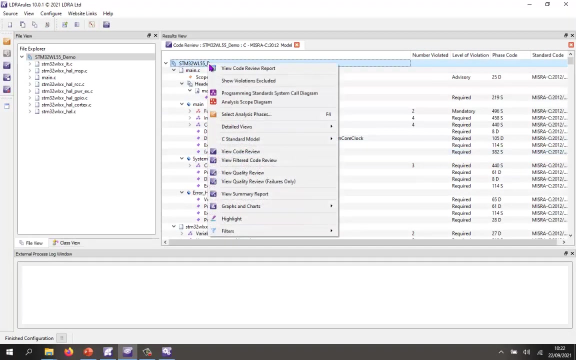 something and we're ignoring it. So what MISRAC says? well, you should put a void cast in front to indicate that you're ignoring the value that's returned. That's fairly easy to fix. What about ones we can't fix? Well, we can justify them. OK, how do we do that? Well, 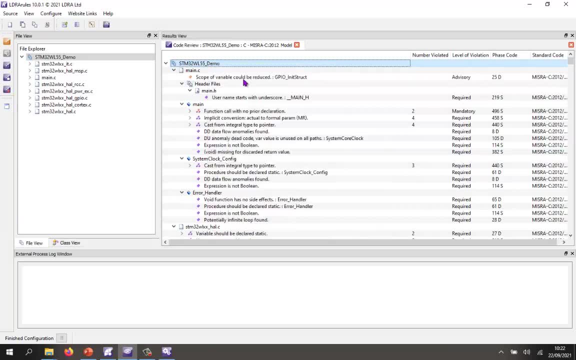 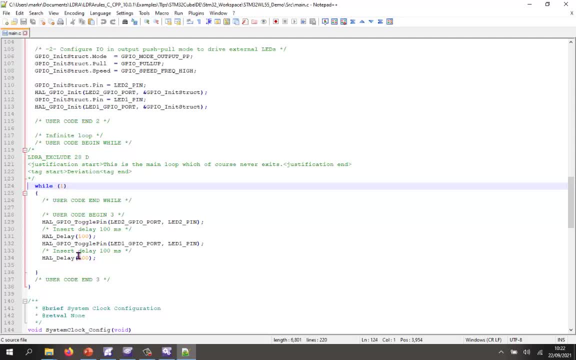 this is going to open up the place where that violation occurs, And here we can see: yes, we definitely have an infinite loop, And so I've put a justification in here to say: OK, this is the rule that I'm violating. And here I've got my description, or my justification. 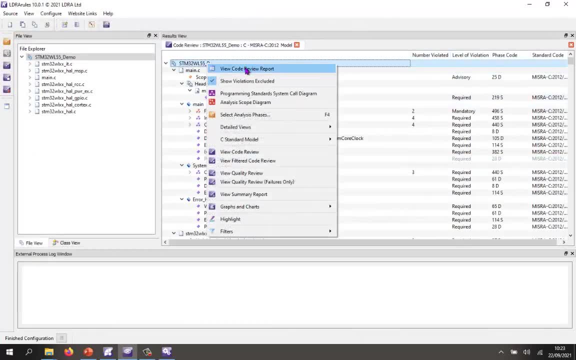 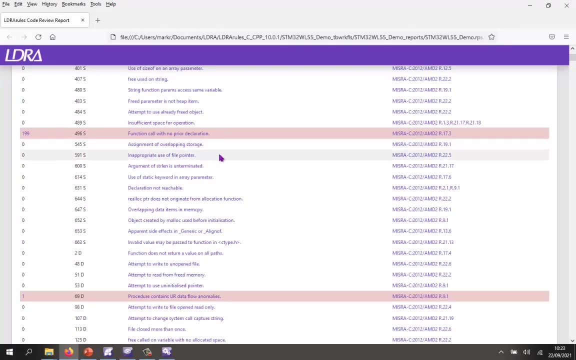 And when we do that, what you'll find is, if I now generate a code review report, we're going to be able to see that inside the report I can see all the places where I have violations. And if I do a Control-F, I can see all the places where I have violations. And if I do, 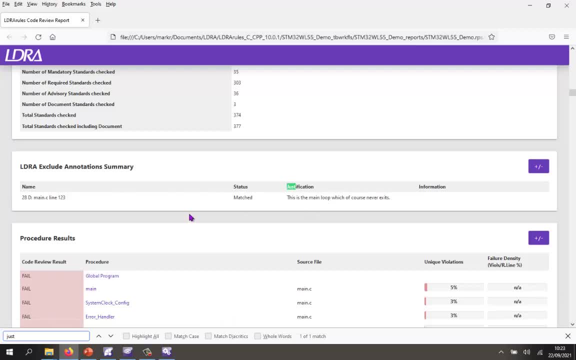 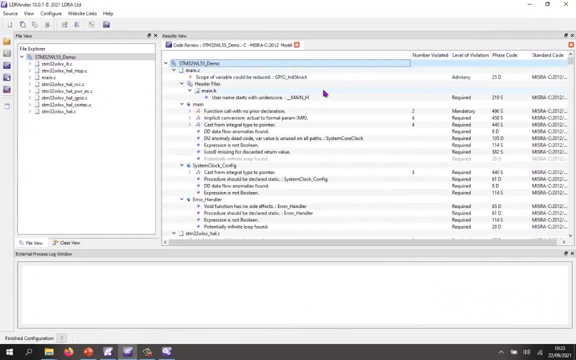 a Control-F, I can see all the places where I have violations. And if I do a Control-F and do a search for justify there, we can see that. there I have my justification inside here. OK, So what about the quality of this code? Well, first of all, let's go and take a look. 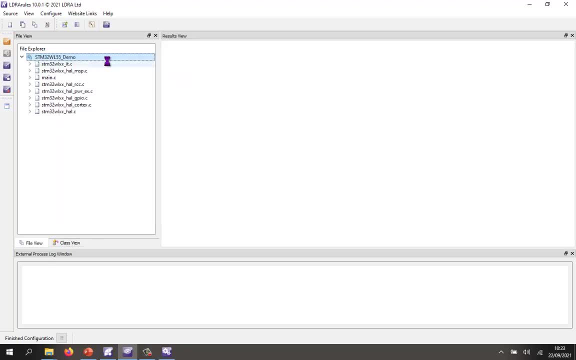 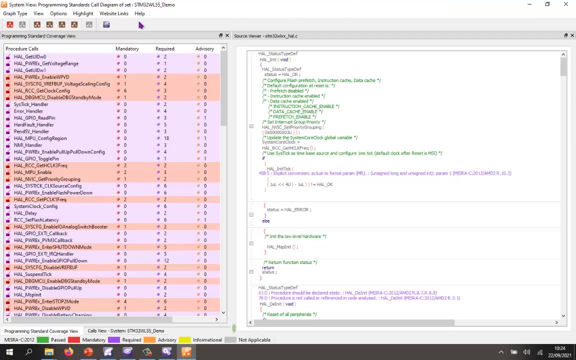 at maybe a programming standards system call diagram. OK, So here we have a call diagram And in this particular case we're able to see all the various violations Here. if I wanted, I can sort and rapidly find where I have the most violations And 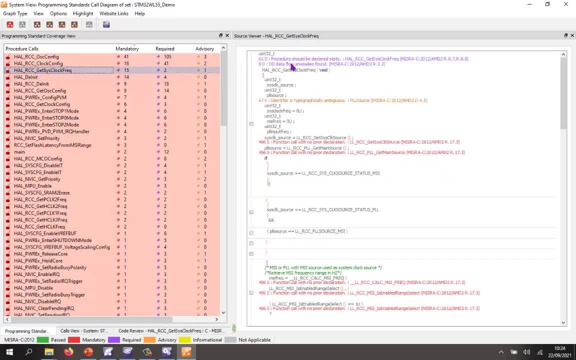 if I click on one of these particular functions here, we're going to be able to see the violations, color coded depending on whether they're required, mandatory or advisory, And again, I can click on any of these and we can see very clearly the violations. Well, I can put this call. 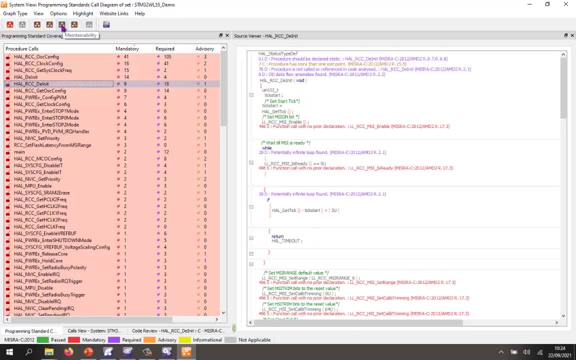 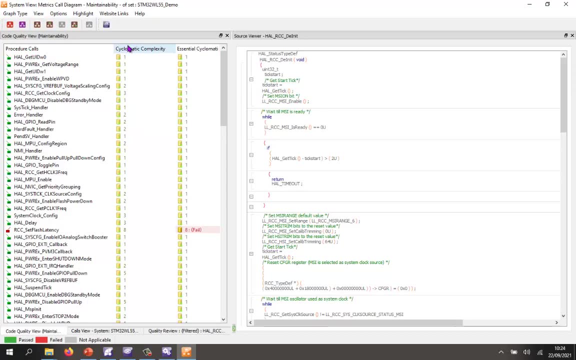 diagram into various different modes. For instance, I can show a mode that gives me an idea of maintainability, OK, And this is where I can see what I'm doing, And, of course, I can also see the violations, And that's where there's two metrics that are interesting: the cyclomatic complexity and the essential cyclomatic complexity. 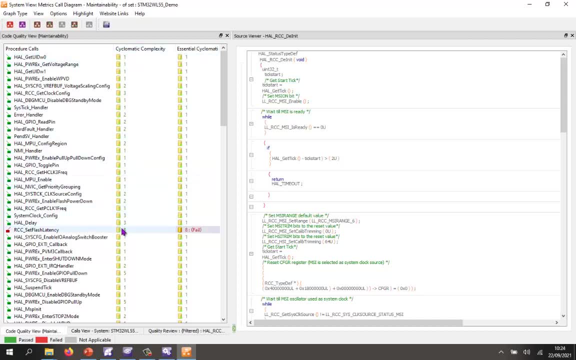 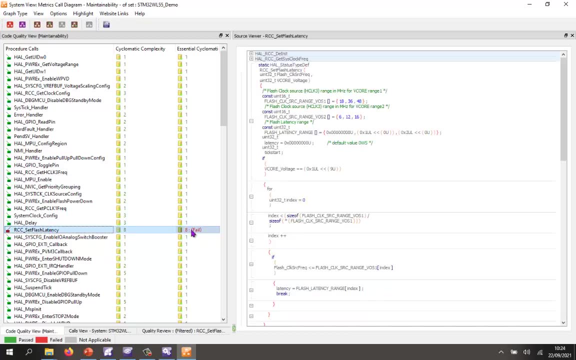 So cyclomatic complexity is giving you an idea of how complex is the function And essential cyclomatic complexity is giving you information about the fact that, yes, this is complex, but you've made it more complex than it needs to be. In this particular case, we can see that somebody's put a break statement inside of a for loop and that makes it more complex to understand. 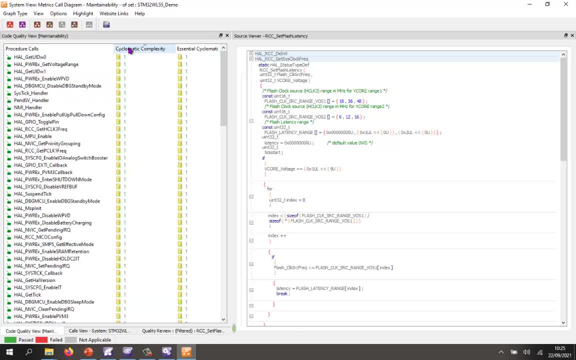 But let's take a look at cyclomatic complexity and let's sort and find the most complex functions. Well, it looks like I must have set a threshold at 25, and we can see we've got two functions here which have a very high cyclomatic complexity. 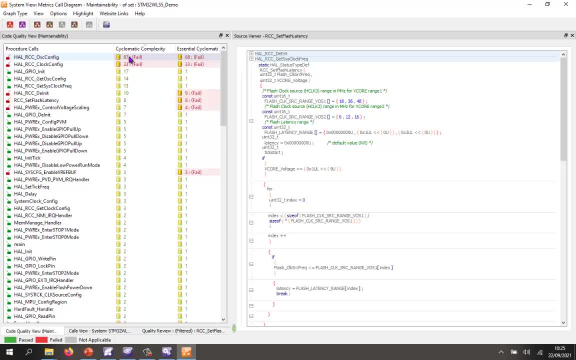 In fact, this one is way too high and really both should be refactored. Well, let's take a look and see what cyclomatic complexity means. Let's take a look at this particular function here and let's view that as a flow. 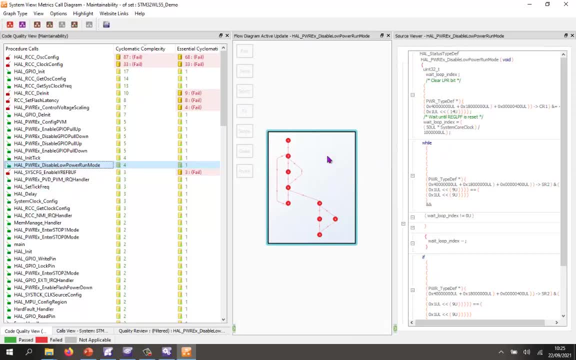 And the flow diagram gives us a nice easy way to understand the flow of the code. So here we can have a block of continuous statements, followed by a branch to another block, Right? so let's take a look at something a bit more complex. 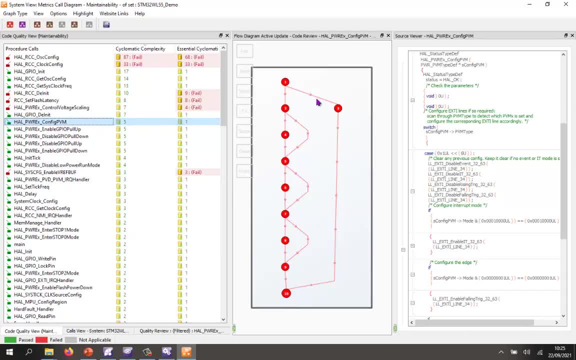 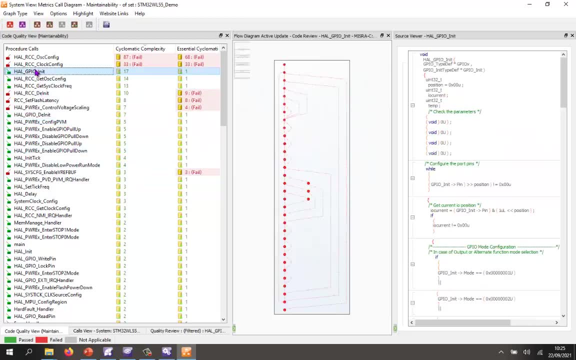 So this one has got a value of 5, and that means there's effectively 5 paths to the code. So we've got 1,, 2,, 3,, 4, 5.. This one's got a value of 17,, and again we can see this is getting rather complex.